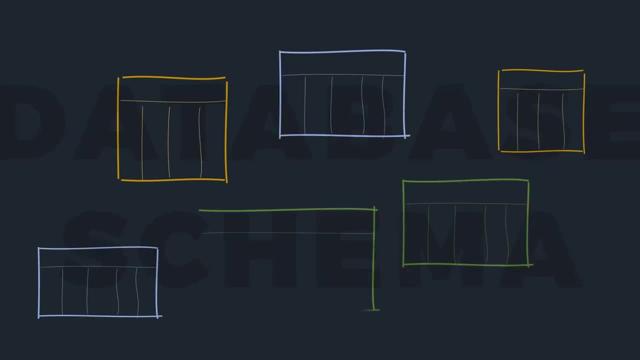 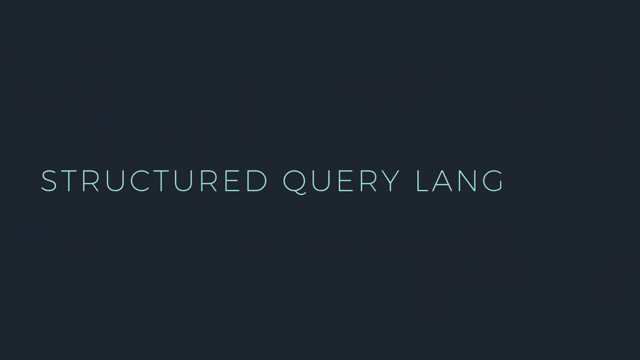 Designing an efficient database schema that addresses business requirements is an art that database professionals spend years learning and perfecting. The structured query language, pronounced SQL, is the standard way to query and manipulate data and schemas in a relational database. That's why relational databases are often referred to as SQL databases. 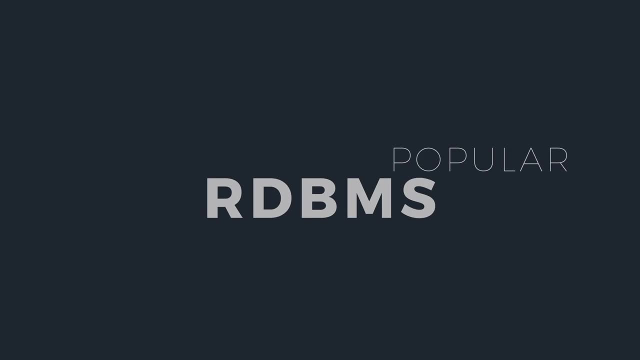 Popular relational database management systems in the market include MySQL, the most popular open-source database. PostgreSQL is another open-source database that is gaining traction in the enterprise. Oracle Database is the oldest and most used commercial database engine. Microsoft SQL Server is also widely used by many companies. 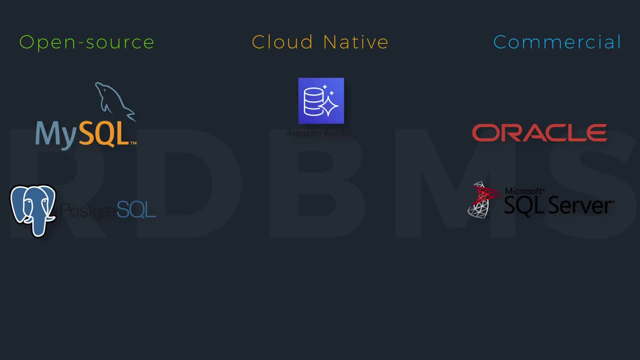 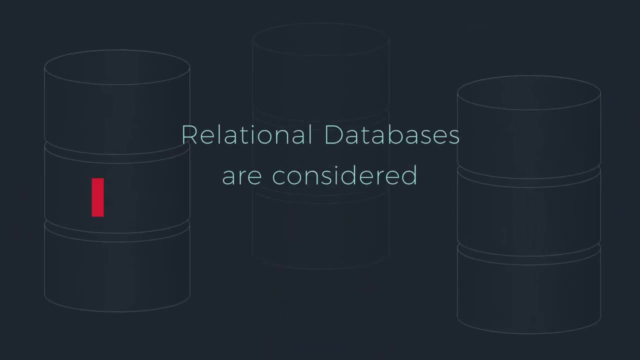 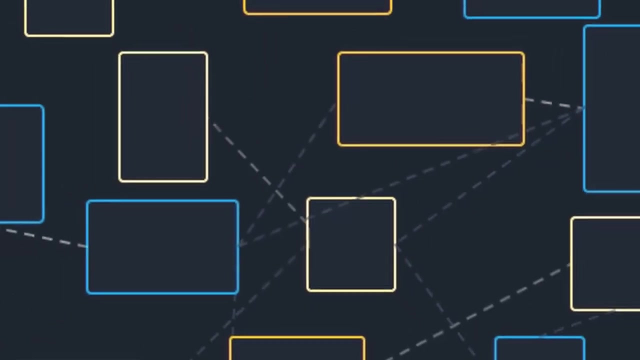 Cloud-native options are gaining popularity, like Amazon, Aurora, Google Cloud Spanner and Azure SQL Server. Relational databases are considered general-purpose databases and are the most common type of databases used to build applications and systems. However, as a database evolves, the high volume and velocity of data, the number of tables, columns and intricacy of relations can become overwhelming. 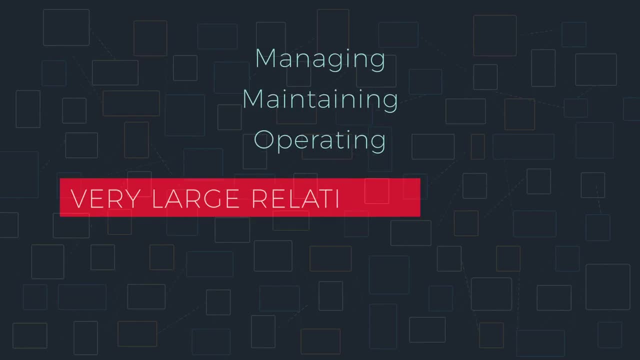 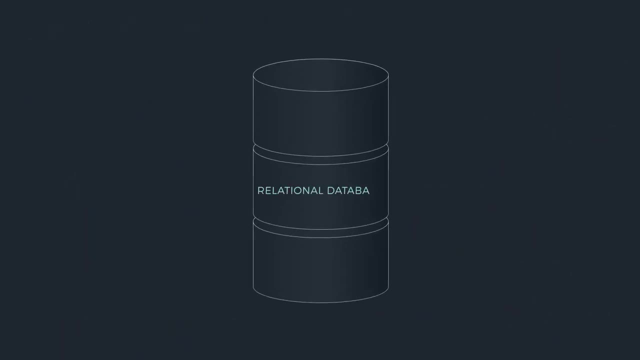 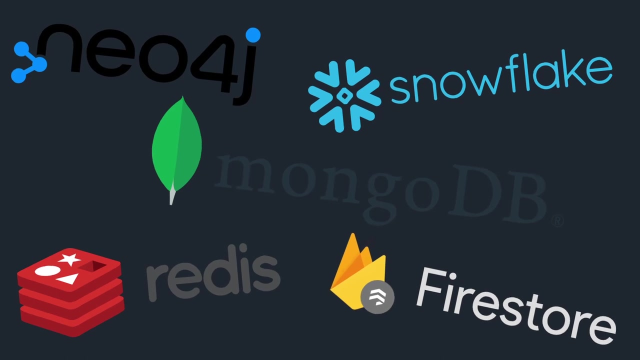 Managing, maintaining and operating a very large-scale relational database can be very challenging and quite costly. In some cases, a relational database may not be the right choice. That's why alternative models gained popularity. These purpose-built databases are grouped under the non-relational or NoSQL databases umbrella. 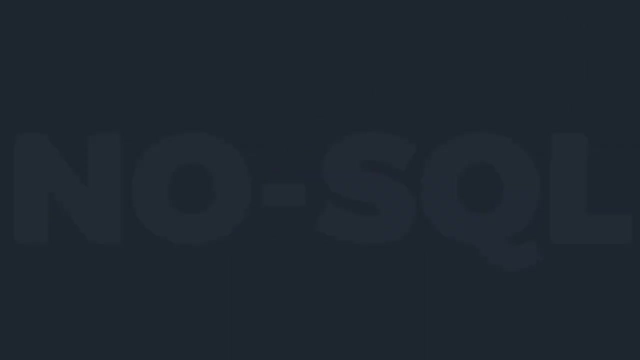 The most common types of NoSQL databases are Key-value databases. Here the data is stored in associative arrays of key-value pairs. This model allows for very fast access to data and is mostly used for data processing. It is also used in in-memory databases like Redis and Memcached. 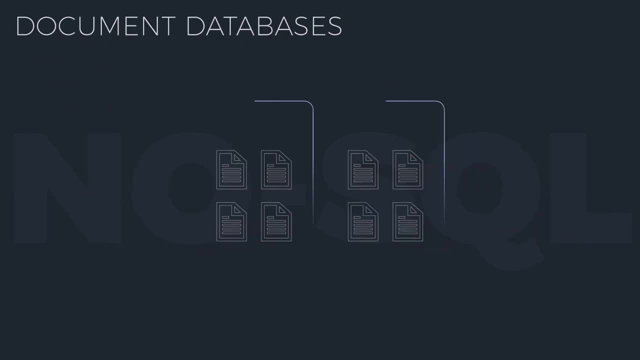 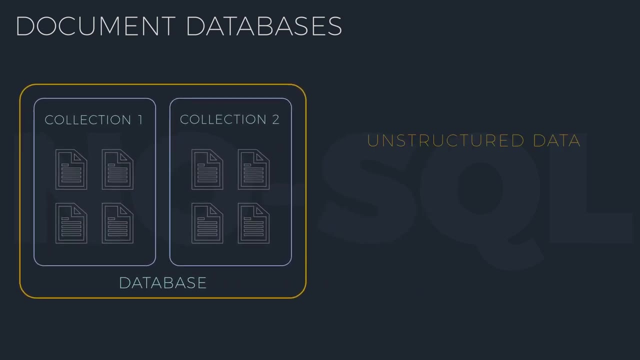 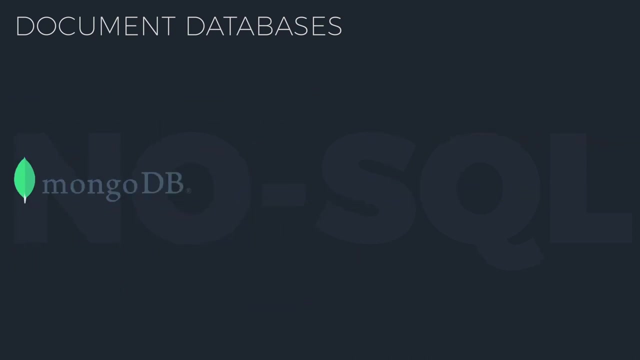 Document databases. Here data is stored as documents, often in JSON format. This model is most suited for unstructured data where the schemas can't be defined or are frequently changing. Popular document database is MongoDB Cloud-native. alternatives include Google Firestore and Amazon DocumentDB.